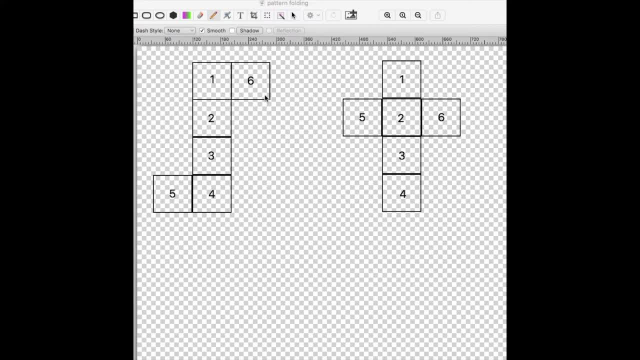 So the very first thing I do when I see a figure like this for a perceptual ability portion is I try to see which two sides of the cube will not touch. So looking here for one, one, second one and three will not touch, They're just going to be opposite sides of the cube. I also know that 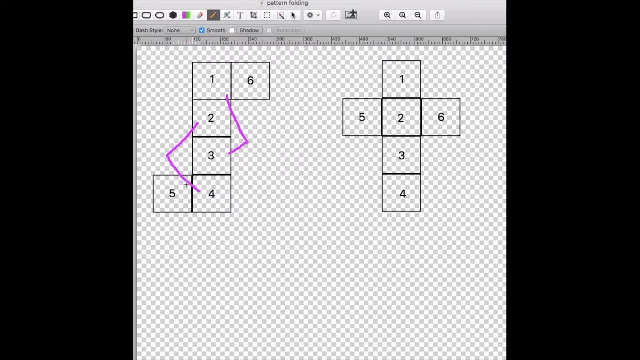 two and four will not touch and six and five will not touch. The reason for that being is like when you have a cube like this, let's say this would be number one and number three would be that back side right there, and they will never touch, and six and five will never touch. So then let's 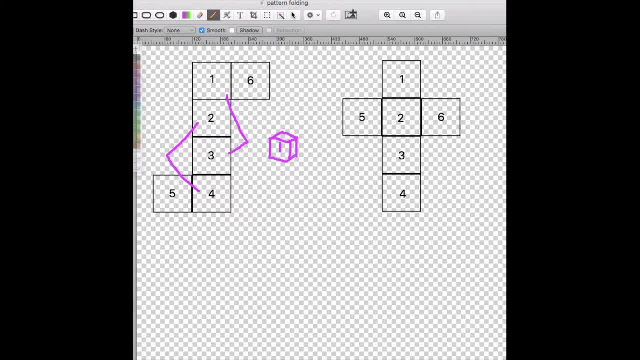 take a look at this one and we're going to do the same thing. We know that five and six won't touch, one and three will not touch and two and four will not touch. So let me do an example problem and show you how you can use knowing this knowledge to eliminate answer choices. 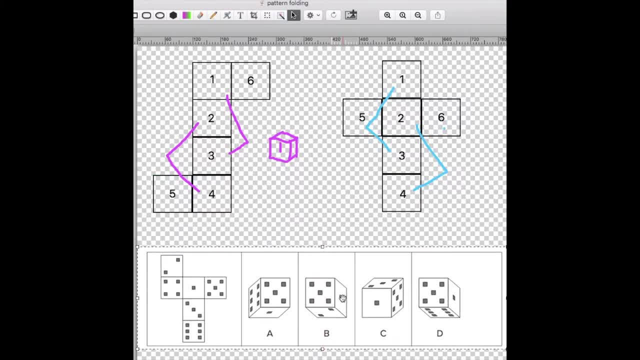 So here is an example from a practice test and we are given our folded up version And the very first thing I'm going to do is I'm going to look at it and I'm going to say, okay, I know that one and six will not touch, So I go to my answer choices right here and I take a look. 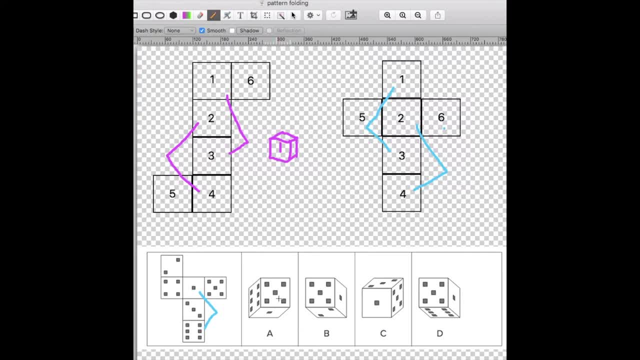 and see where one and six are touching those sides. So I see that one is right here and six is right here, but I know that like an example here they shouldn't touch one and six. and then there's one and six right there, So we can cross out. answer choice a, then I'll go down the line. 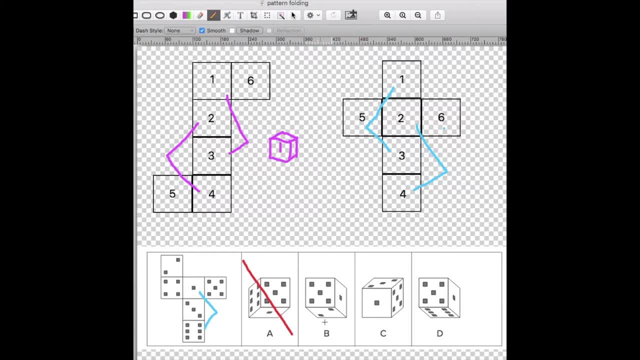 and see if there's anyone else. one and six: I see a one here, but I don't know where the six is. I can't not eliminate b In c. I have a one, but I don't see the six, so that could potentially be the correct. 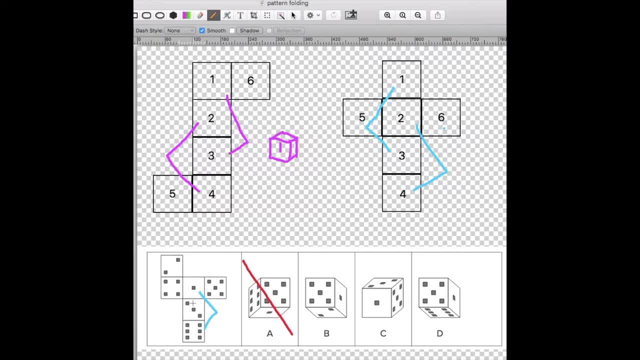 answer And in d I have one and six touching, but once again, they should never be able to touch. They are on opposite sides no matter how I turn the cube around. So I can eliminate answer choice d And just like that, within a few seconds I was able to eliminate 50 percent of the answer choices. 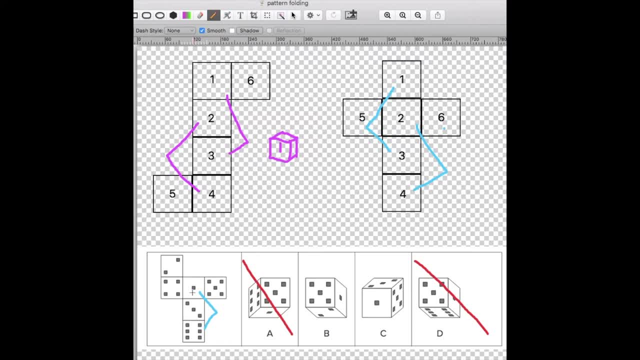 So that's awesome. So now we're going to go to the next thing. Usually I just go through and I go: okay, four and five will not touch, because of course they're on opposite ends. again I have. I don't have a four here, I do have a five. That doesn't help me. I've got five here, I don't know where. 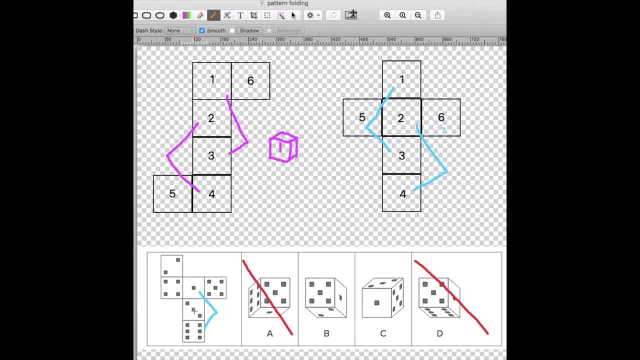 four is. That doesn't really help me, And then I'll quickly do it for this. I know that three and two will not touch, because two could be spun around right here and go right there. So I know that they're opposites and they will not touch. So I quickly check and I go three, I don't see a two. 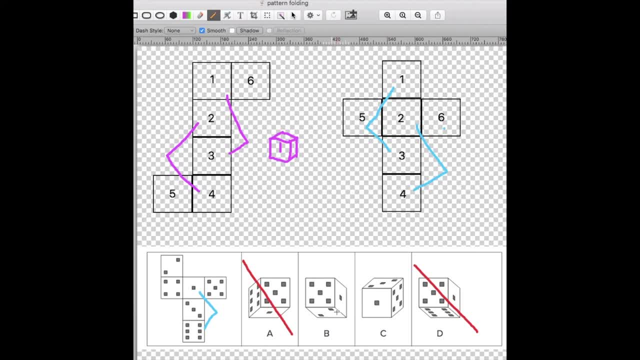 three and I don't see a two. Still, with that quick technique that took, like I don't know, three seconds, I was able to eliminate two answer choices. So now I'm going to take a look at b and c a little bit more closely. 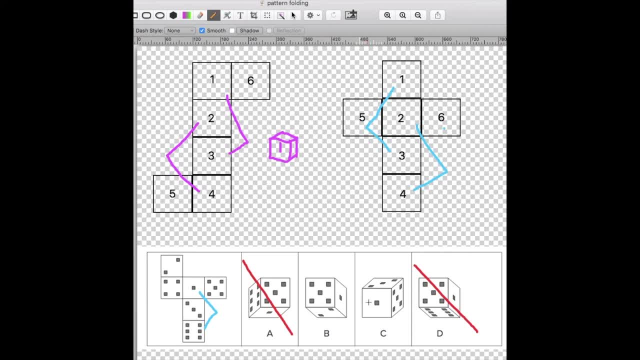 And I'm going to take a look at it and I'm going to say, okay, which one should I look at? If I start with b, I've got five right here, but one is on the opposite side, So I'm going to have 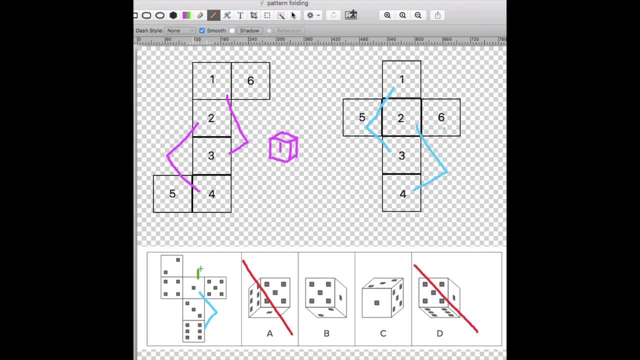 to like think about flipping this whole figure, like give it a 180 turn, And that can be hard to visualize, It takes a little longer. So I'm just going to go ahead and take a look at c before I do all that visualization stuff. So in c, one is our front face, Here's one, And we know that. on the right, 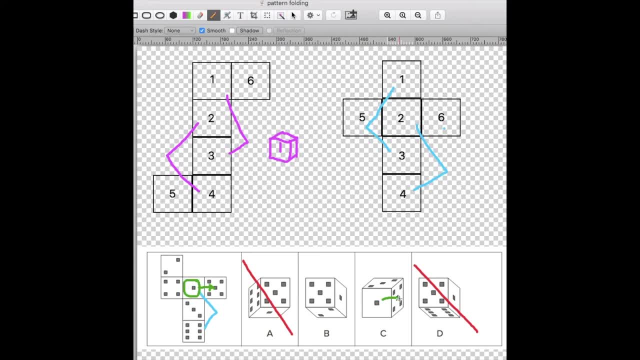 side of one, we have five, And that's exactly what we have here. That's good, And above it we're going to have this, So that's going to flip there, And above it we should have. let me take, show you guys, what we should have. So once we flip that, 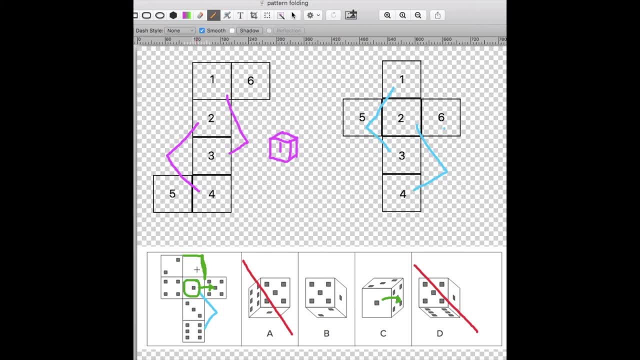 that's the square, this will go right there, that's our dot and this would go right there. And we see that we should have two above the one. straight above it should be two from this flipping, But we see a three, the threes actually below it, not above it, And we know that that is.